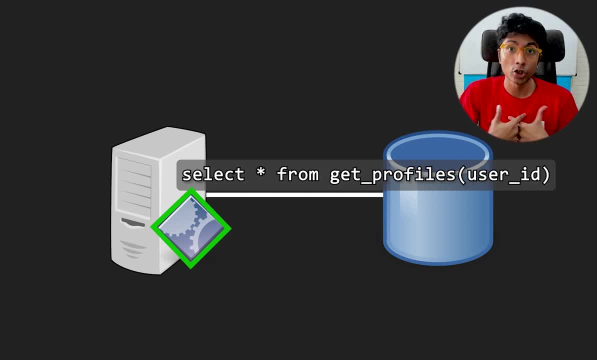 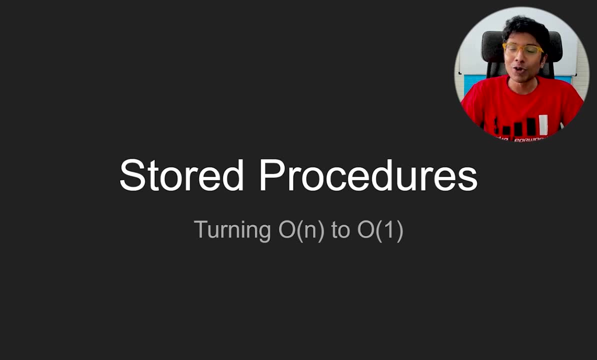 you'll say, let's say, get profiles, and which kind of profile should this user be able to see? So user ID will be the input and the output will be all of the profiles that I should be able to see. So when are stored procedures actually useful? Now let me share with you a real 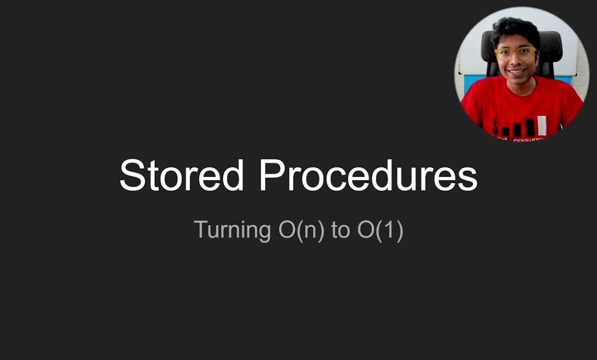 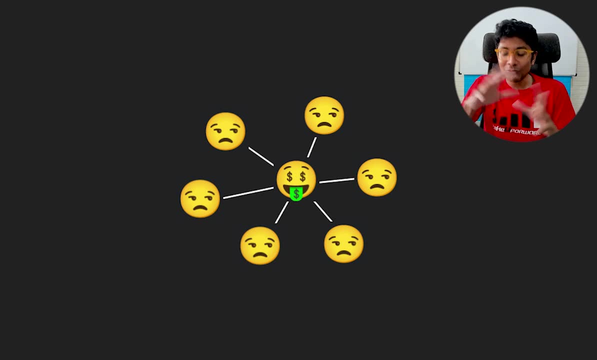 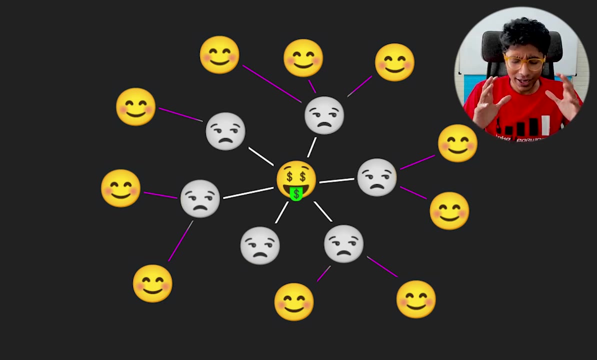 world example. This is way back in 2015.. One of my friends was trying to build an app for personal loans and the idea was that you might have run out of your close relatives, and everyone but relatives of your relatives may still be willing to give you a loan. So as crazy as the idea. 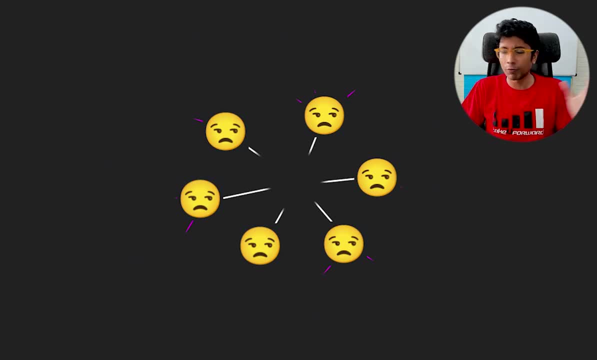 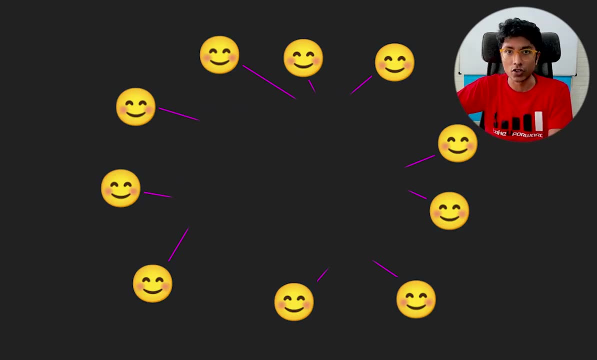 sounds. the basic idea is very simple. You have a set of friends, a set of people who you know, So they are your connections, first level connections, And then there are second level connections, who are the connections of your connections, So one transitive relationship. The idea here is: 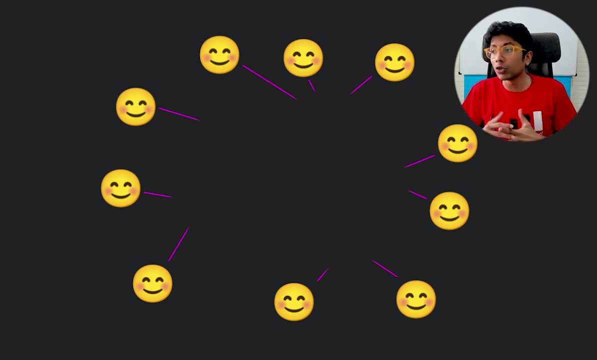 that if you can find that larger circle of friends, of friends, then you can suggest a loan to be given to you. But the problem was that when they were trying to run this query it was taking too long. It was taking, I think, about an. 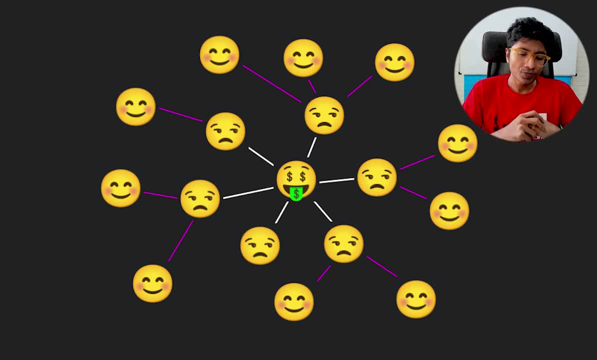 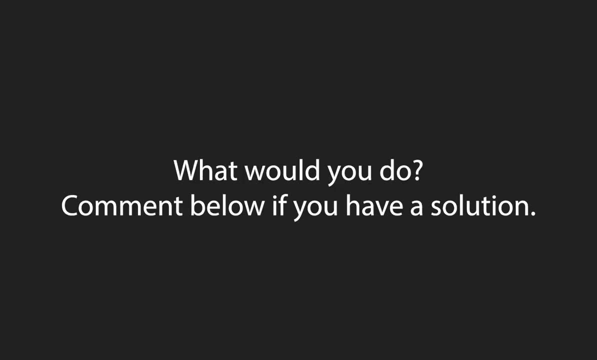 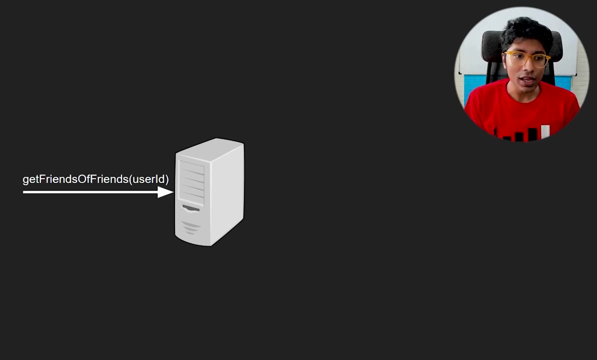 hour or something in their database. So they came to me and they asked me for an algorithmic optimization and this is what I suggested to them eventually. So they had a server and the server was getting this request of get friends of friends, with a user ID. Then they were making a query to the database to find 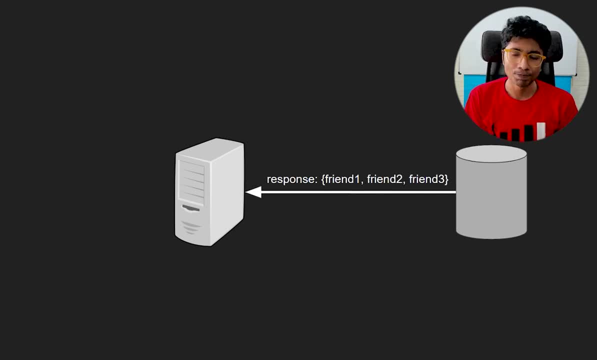 all the friends of this user ID. This is the original user. let's say me Now that was returning a response of three friends- Friend one, friend two, friend three- And then what is happening is iteratively: we were going over the friend list and getting 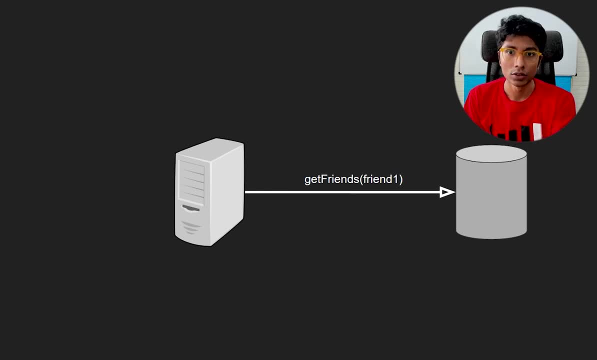 a direct connection. So what's happening now is the second order response is going to come back And this is happening, let's say, for one person. one person had around 50 or 60 friends. You would be running this 50 or 60 times. 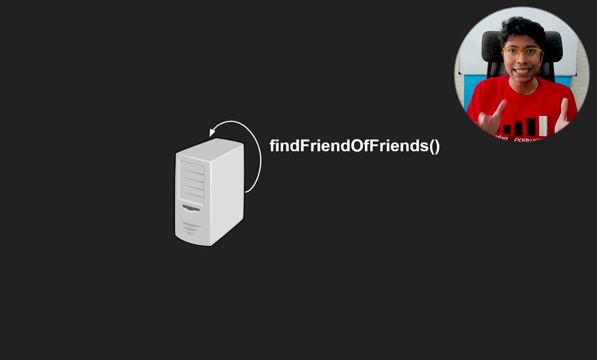 Finally, when all the friends were together, they were put into a single set and then, after you know, removing duplicates and putting them in a sorted order, there would be a response. But the response, as you know, was taking very long. it was about one hour. So my first suggestion to them was to use a optimized 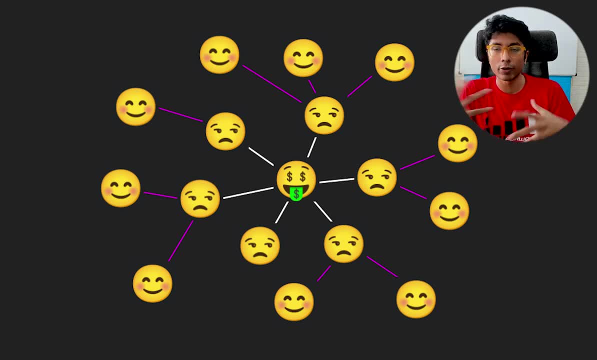 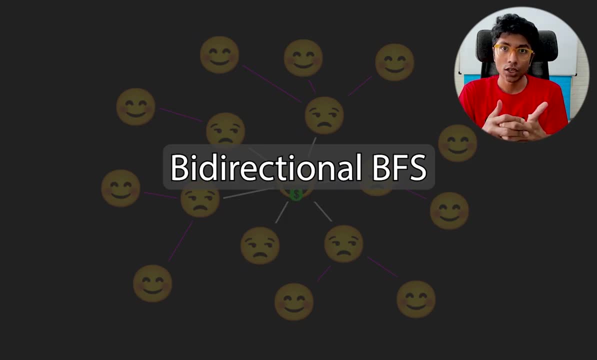 algorithm for this. This is a graph and the graph has a set of nodes. You are basically trying to do two traversals, so I suggested to them to have a bi-directional breadth-first search. Here. you have nodes on each side, friends, and 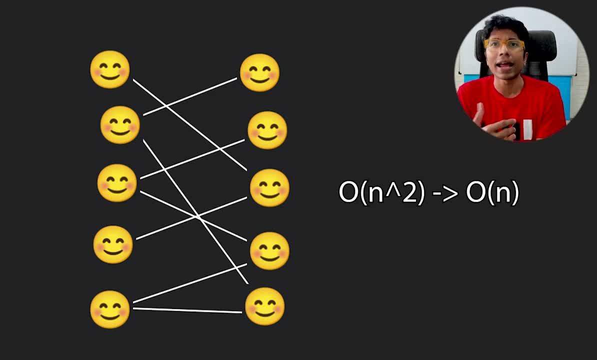 friends trying to connect with each other. Instead of an order n-square query, this becomes an order n query. This is all theory, though, because in practice, it didn't change the runtime. The runtime was still one hour, and that made me feel a lot of surprise, Like I was like what? It's still as slow as ever. I asked them: 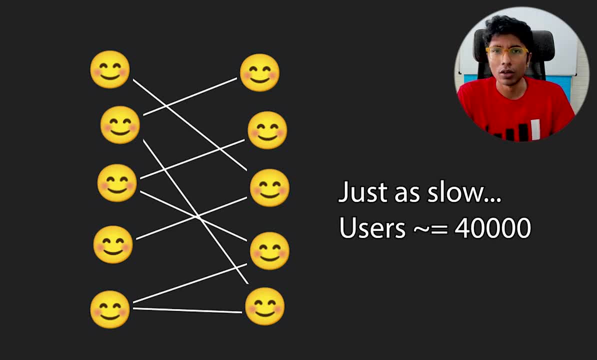 the size of their inputs. The size of the inputs were very small. It shouldn't really have mattered. Everything should have happened in one second. I think the number was something like 10,000 or 1 lakh, which is 10 raised to the power 5.. So BFS. 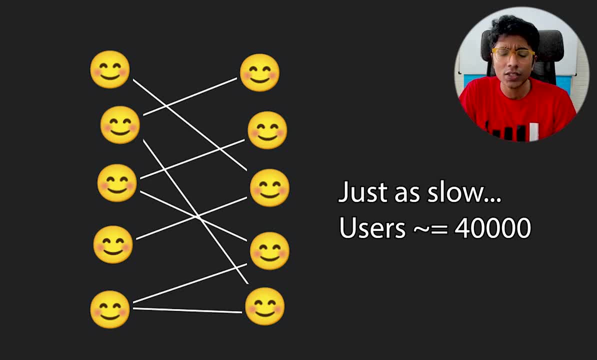 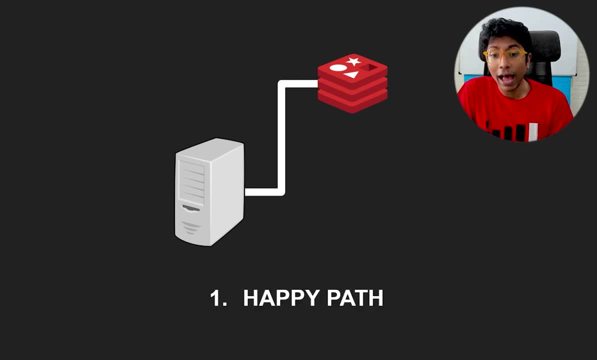 should have worked. It didn't work. That's when I suggested that, hey, why don't you just cache the results? This was super effective. It worked out really well. There was a happy path where you would just query for your friends of friends, as a user, and you would get a. 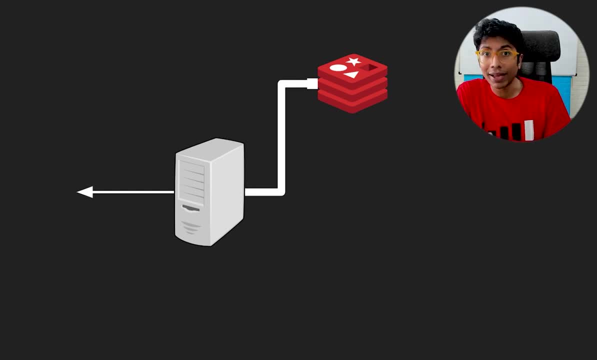 response in a second, So their average response time actually went down to less than a few minutes. The only problem, though, was server restarts. Whenever there was a server restart, we used to have a cache miss, because the cache would get evicted and we would have to fetch from the database Again. that would take about an hour to respond and one of the solutions was in the night. at 2 o'clock every night we can just restart the server. Any kind of deployment will be done in the night. Any kind of cache refreshing will be done late in the night. That was their. 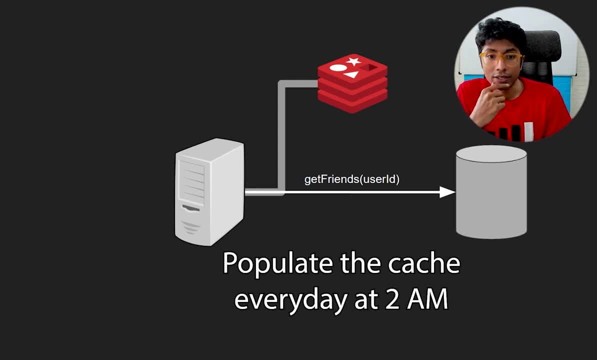 idea. The other problem which is over here is that if your server crashes, then if it's an unexpected crash, then you have no choice. You have to go to the database and put the entries. My solution here was to use a global cache that the 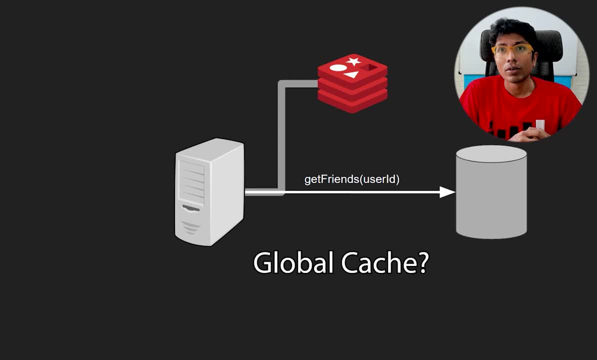 cache does not get scrubbed out. but this also didn't feel good because you didn't have fast updates in this cache. One of my friends at this point said that hey, instead of a global cache, why don't you have a global cache? Why don't you have? 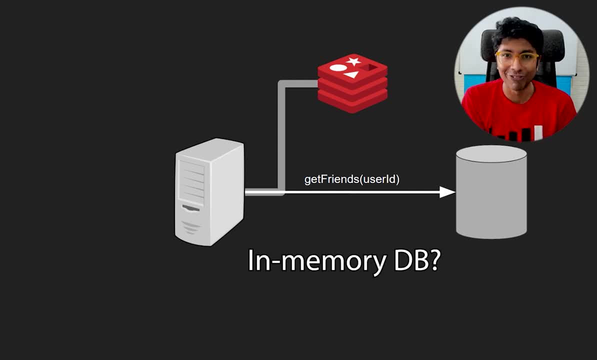 an in-memory database itself, So it's like a cache after all. and that's when it struck us something is terribly wrong With around 10 raised to the power 5 entries. if it's taking an hour to run a BFS, that makes no sense. Even then, hardware was. 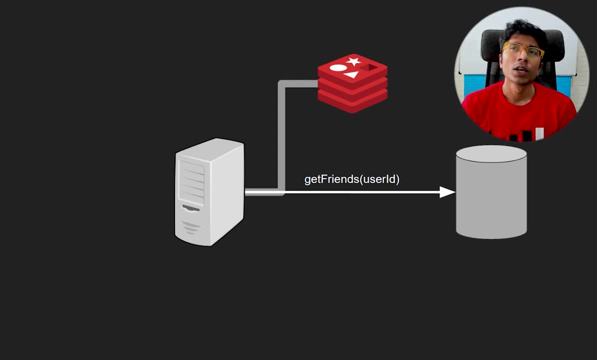 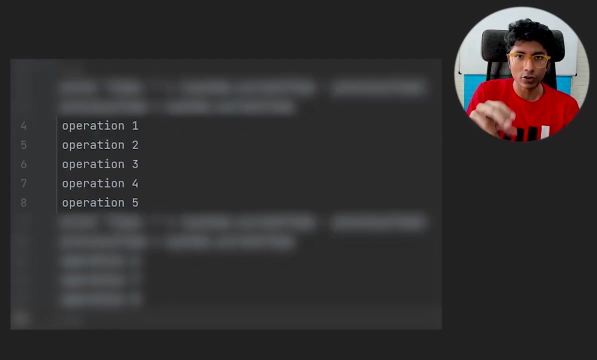 enough to run 10, raised to the power, 7 queries per second. So here's when we started thinking, finally, and we start tracing the problem. So we started, you know, writing down SOP LN statements after pretty much every four or five lines of code and we realized where the problem is occurring. Our first query to the 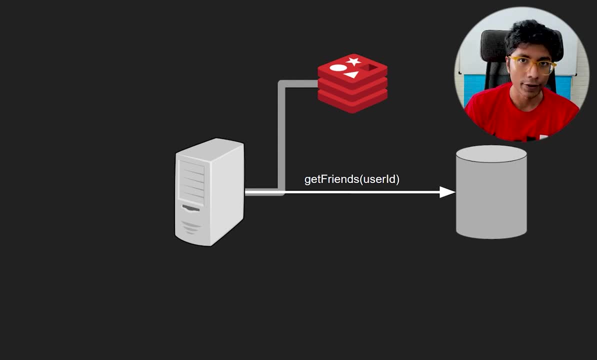 database was get friends user ID. This would take about one second. The response would give us friend 1, friend 2, friend 3.. In fact we would have hundreds of friends for certain cases. Then we would make another query and this would take about. 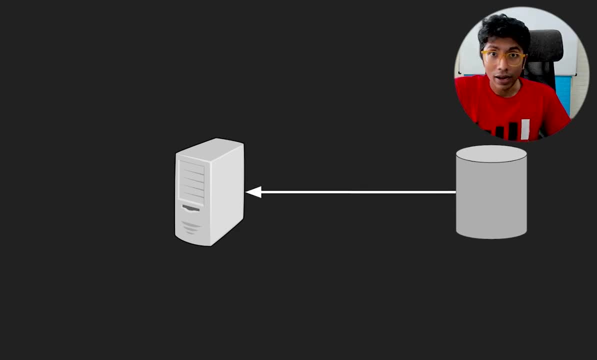 one second to respond, And then again and another second. So what was happening is that we were making a cross-continent call. Every time this query was being run, we were hitting a database in the US and our server was in India. The second problem was that we 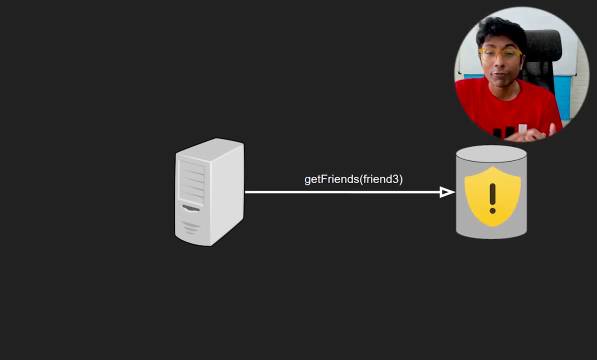 were making too many requests to this database. The firewall found our activity to be pretty suspicious, So it started blocking these many requests coming in suddenly from from one server in India. So it's strange. I mean, maybe the firewall didn't need to behave this way because it was a server of the company. 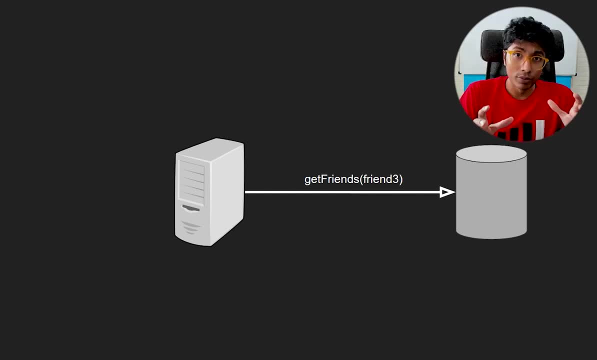 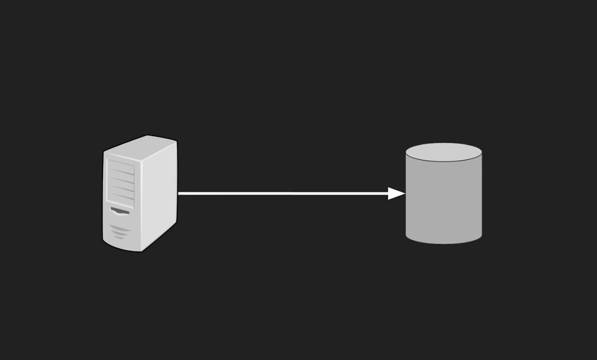 but it happened. However, it's good because by making the runtime so large, obscenely large- one hour- it actually helped us focus on what is the code problem, which is these many network calls, And the idea came up then: stored procedures. You know why don't we just run this entire algorithm of breadth first? 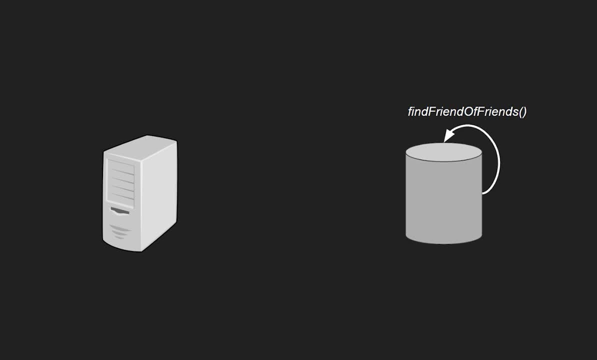 search in a stored procedure. So this will be a bunch of SQL statements. You do an inner join on the friends table and you find your friends of friends that way. Then you return a response and everyone is happy. This worked out. This worked out really. 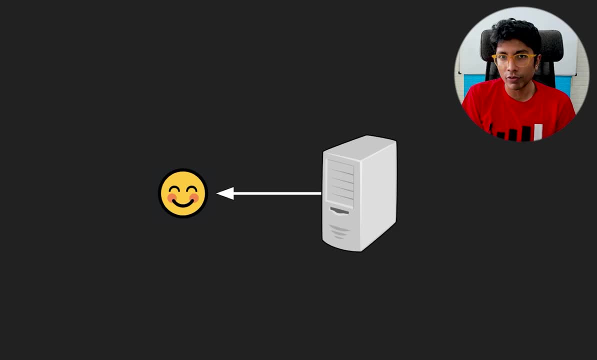 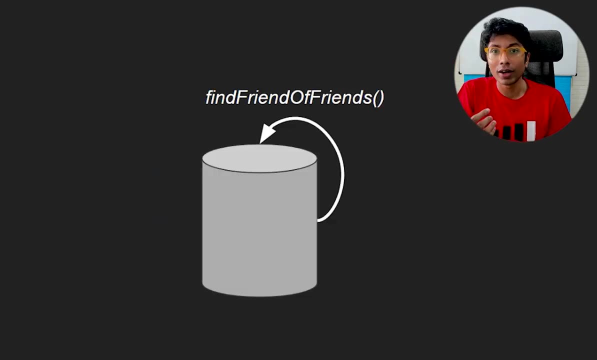 really well. Our customer was pretty happy when they saw that we were able to give responses in a second. They asked us not to implement the cache. They wanted completely consistent responses. Sometimes when you're talking to people who are, let's say, not very techie and you tell them that, hey, sometimes the 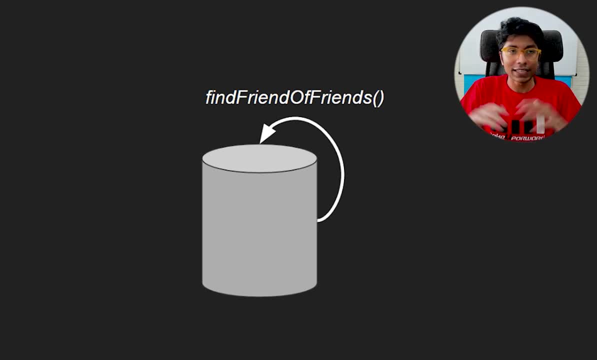 response may not be what is being reflected in the database. They instead tell you: just simplify things, tell me that sometimes things can go wrong and sometimes things will go right. The moment I make a change in the database, it should reflect in the front. 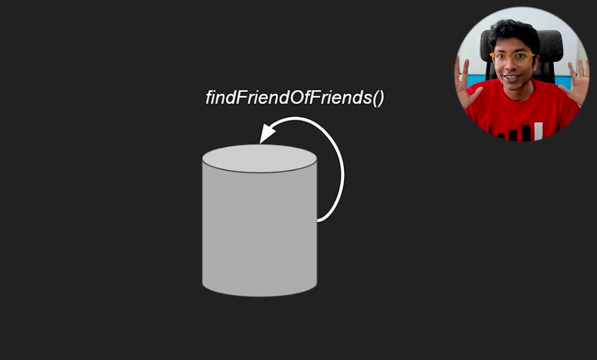 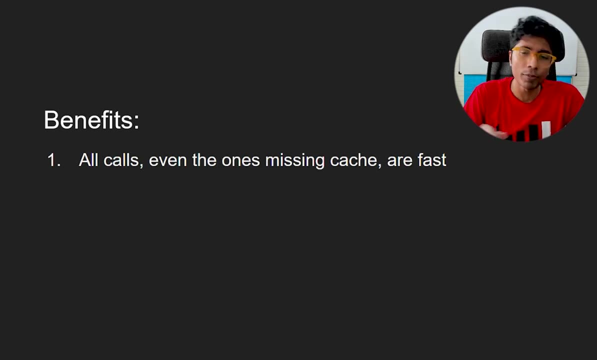 end, and so this is the kind of solution they wanted: No caching, just stored procedures. As you can see, there are many benefits of using a stored procedure. The first one is that there is a certain uniformity in performance. Whenever you're saying, 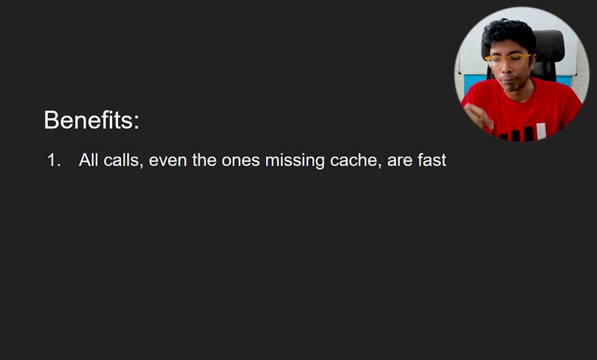 get me the friends of friends. it's always going to take you. almost the same time. You don't have any set of heavy users who have millions of friends, or you don't have light users who have just a few friends, and so you optimize for each type of user. No, that's not. 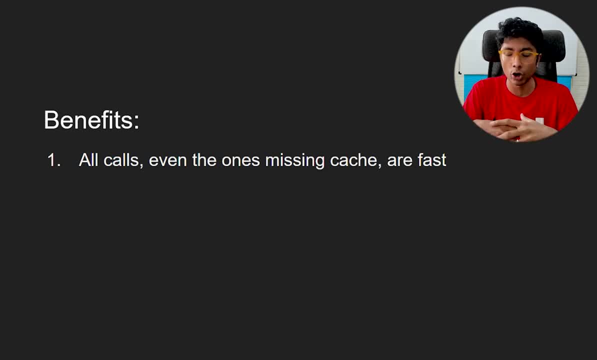 necessary. Just run one query. encapsulate all of that complexity of that logic into a single stored procedure. run that in the database, get a response. It's almost always going to take the same amount of time and the scaling also. that has to be done. 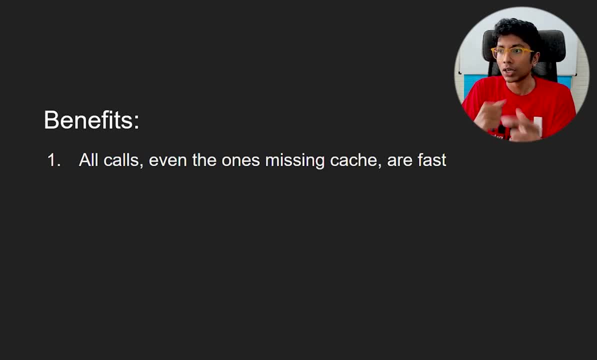 is dependent on that single encapsulated operation, not on a bunch of queries that different servers are making from different places. The second thing is that you don't need any external two-phase commit to be done if you want the operations to run atomically. 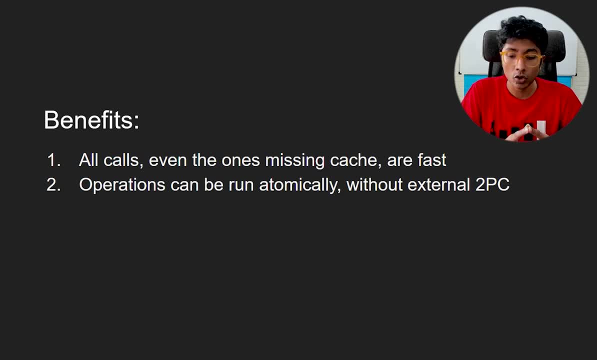 Many databases offer transaction support asset guarantees, so you can have atomic operations running and you can roll them back easily in the database itself. You don't have to manage that through the application. The third point again is very similar. Consistency guarantees in an application are usually harder to enforce. 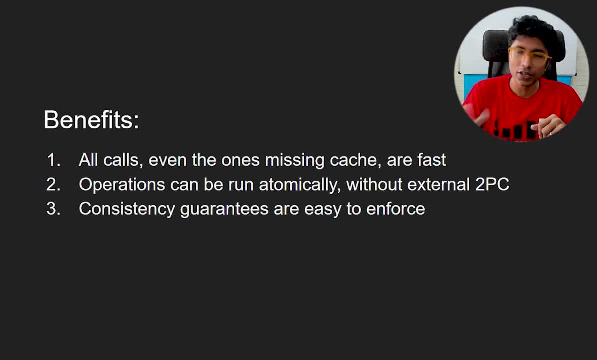 Databases are specialized for this. You can have read committed or serializable isolation in the database itself. Run the stored procedure. everything will appear in the way that you want it to appear. The fourth point is quite interesting. You may have a strong. 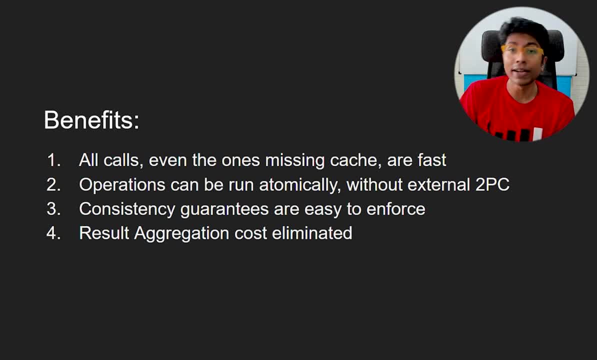 connected network of friends. Each friend is a friend of everybody else. If you have 50 people that would be roughly 2,500 total results that you would get from the database after 50 queries. But if you run the query in the database, 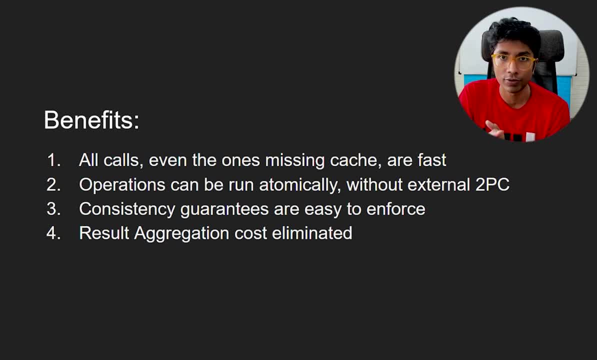 you're going to just get 50 results back, because it removes the duplicates by itself and filters through things by itself. The network cost here is also lesser. Finally, number five, of course, is that you have fewer round trips. It's not like one query instead of 50 queries. This is probably the biggest benefit. 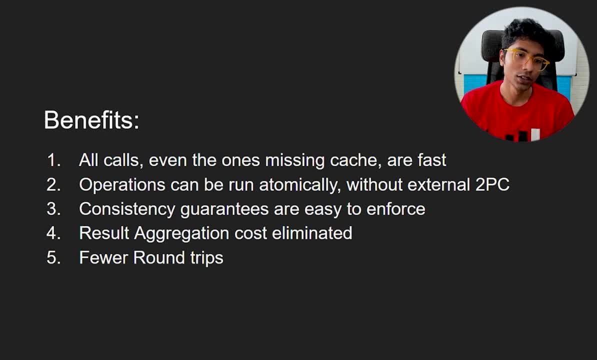 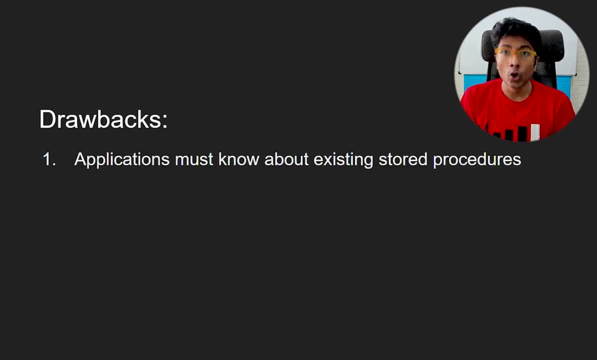 and the most common reason why stored procedures are used. There are also certain drawbacks to stored procedures. The first one is that the application must know and also create a stored procedure. So either it's a database administrator, somebody with the permissions to go and create a stored procedure, will go ahead and do that. 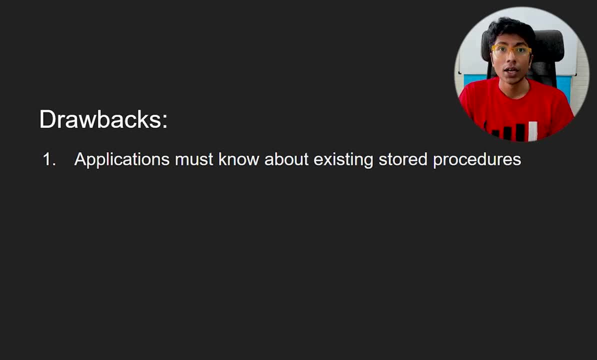 And then you have an application engineer who's going to be calling that stored procedure. They can't really make easy changes to that database. if it's you know, if there are permissions behind the database or if they don't know how to go and change the language of the database, this is going to be a problem. 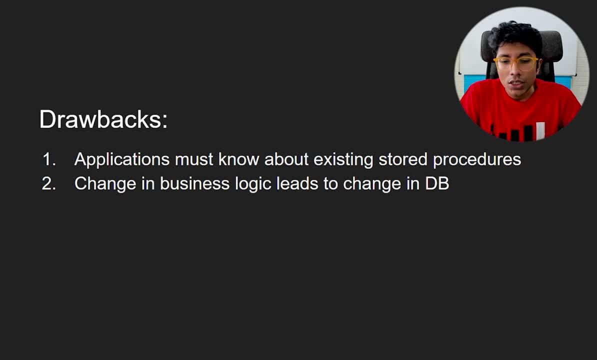 The second thing is your application specific or business logic changes start moving into the database. So this is usually done by the application engineer, who are going to write really bad code. It's going to be difficult for them to maintain the SQL standards that are set by the DPA, or the DPA will say: okay, I will do it for you. 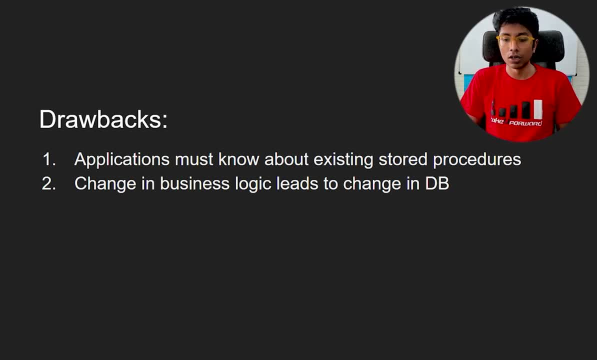 but I'll do it after three days, So development time becomes uh long. It's also hard to read these stored procedures for an application engineer. It's hard to debug for them because when they look at SQL instead of, you know the language that. 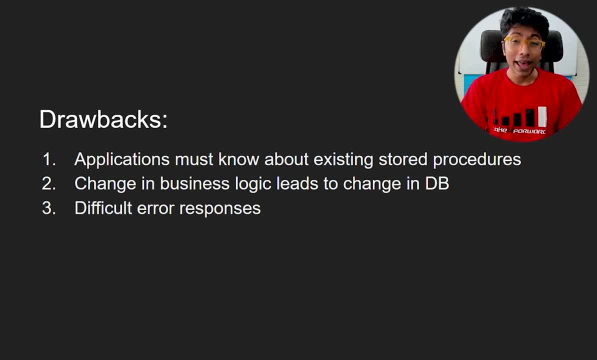 they're comfortable with. it takes them more time. Also, error responses get really different. in an application, It's easy to identify where things went wrong and return the right error code with the error message. But in a DB, when things go wrong, uh, it could be anything. 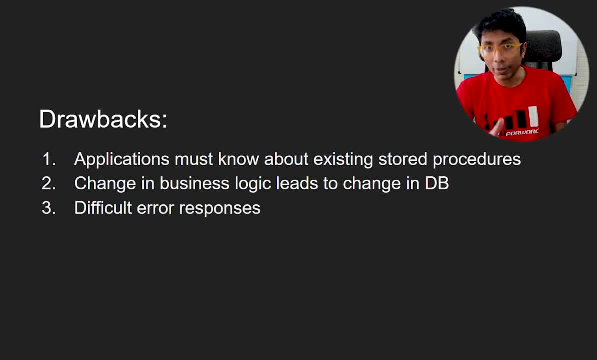 If you get SQL error codes, so the database will not be able to caught up in that. So this is: those have to be mapped into application error codes and that is tedious, It's not easy to do. After a certain point in time it starts getting tiring because you 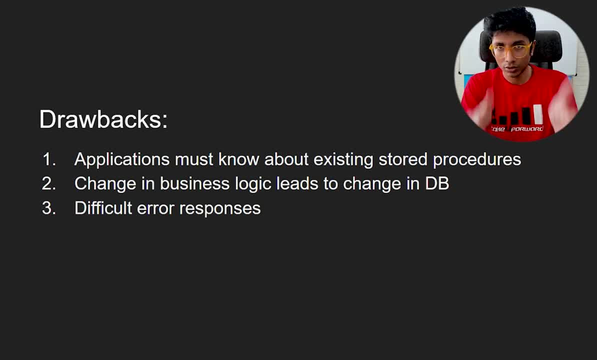 have to have this SQL doc next to you and the application doc, HTTP codes, SQL codes and the mapping. And the absolute final point is that this is database specific, So some DBs will offer you Java support. some DBs won't, If you change. 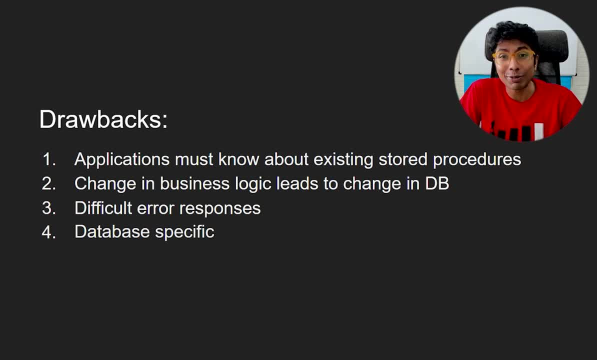 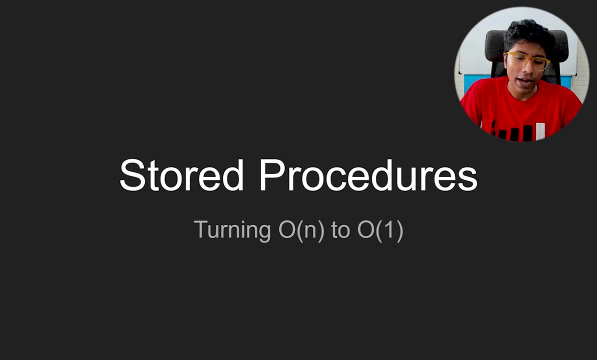 your DB, which is, god forbid, you don't. but if you change your DB then you have to write those stored procedures again, While in an application you just copy-paste code. In a DB it's a little more tedious. So that's it for stored procedures. It's a very simple concept and it helps a lot.